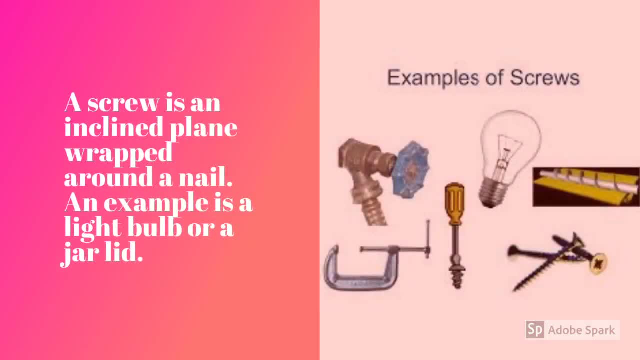 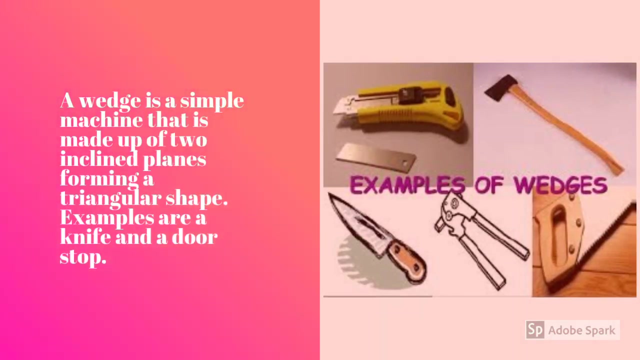 An example is a steering wheel or a doorknob. A screw is an inclined plane wrapped around a nail or a cylinder. An example is a light bulb or a jar lid. Anything you have to screw on or off is a screw. A wedge is a simple machine that is made up of two inclined planes forming a triangular shape. 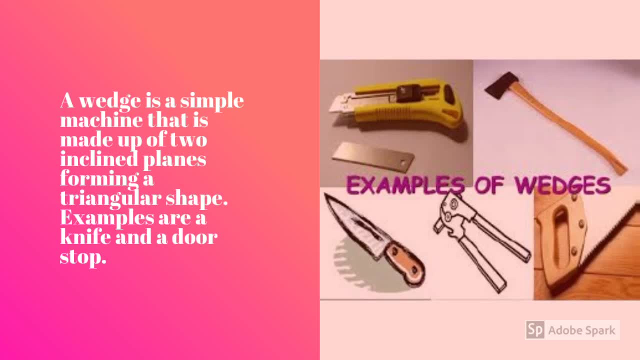 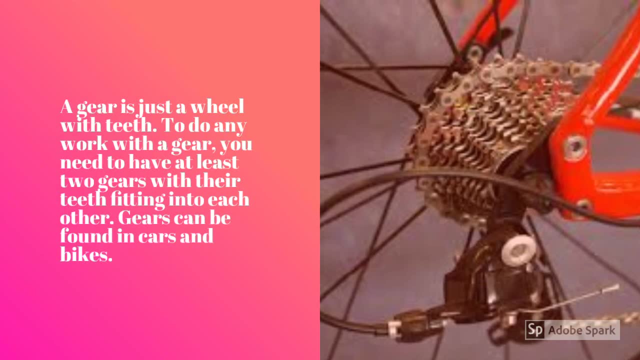 Examples are a knife and a doorstop. Anything sharp is usually a wedge. A gear is just a wheel with teeth. To do any work with a gear, you need to have at least two gears with their teeth fitting into each other. Gears can be found in cars and bikes. 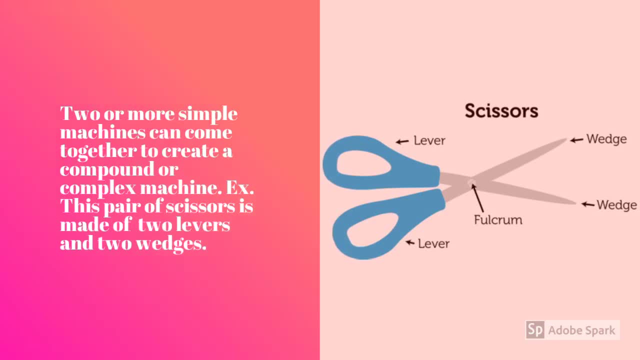 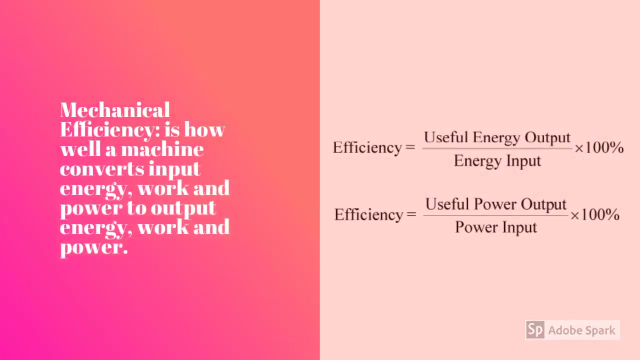 Two or more simple machines can come together to create a compound or complex machine. Example: this pair of scissors is made of two levers and two wedges. Remember, wedges are also inclined planes. Mechanical efficiency is how well a machine is designed. 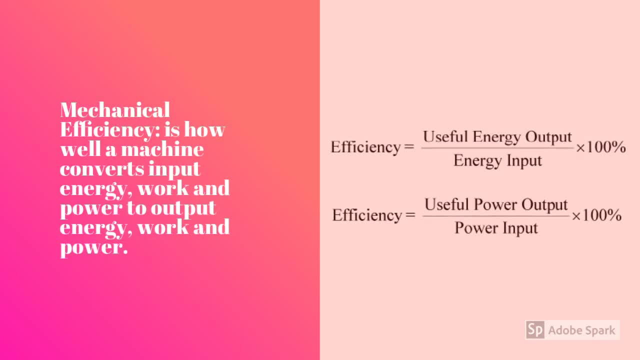 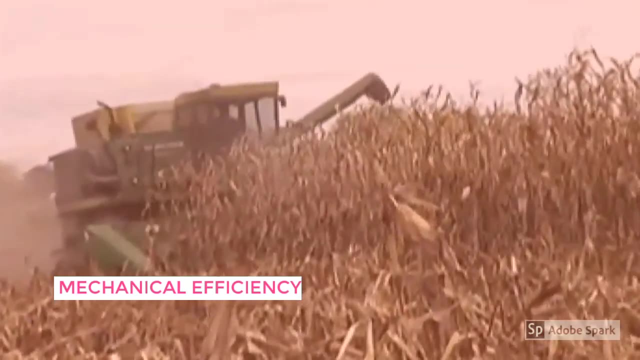 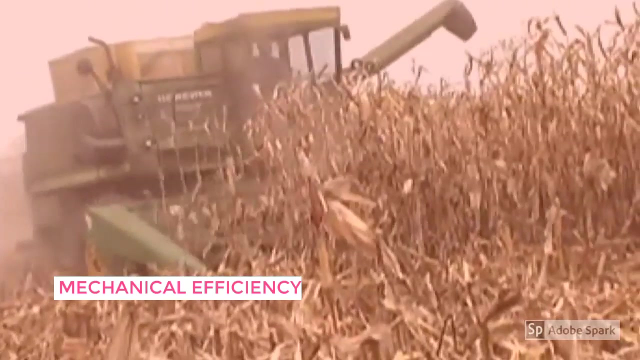 It is a matter of precision How well a machine converts input, energy, work and power to output energy, work and power. Unfortunately, most machines are not totally efficient. Efficiency is based on a comparison of the amount of energy put into a machine and the amount of energy it supplies. 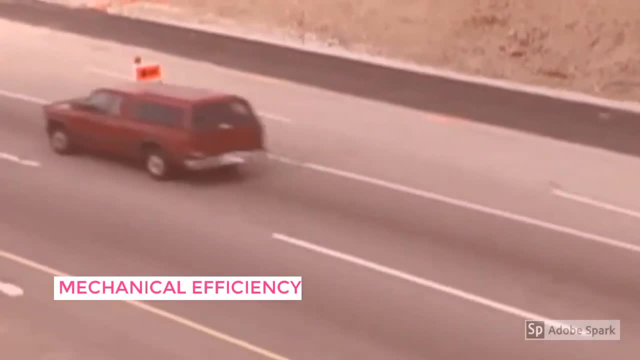 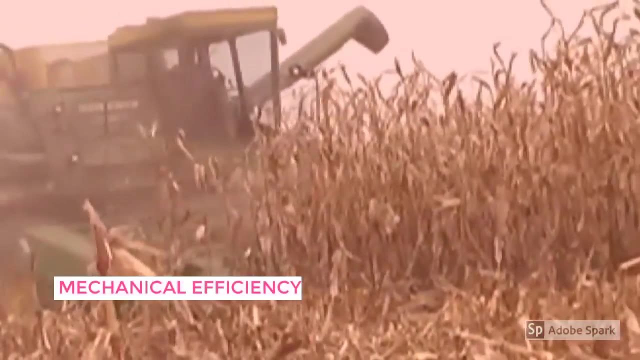 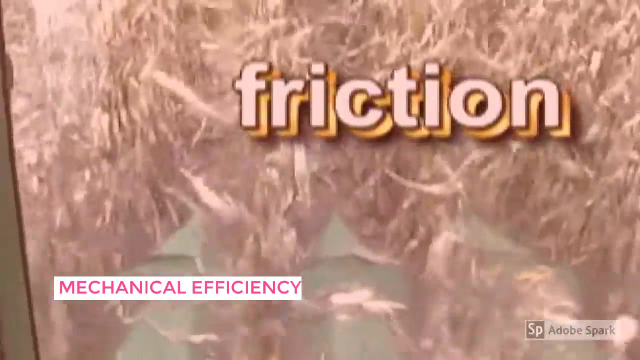 Cars are only about 25% efficient because a great deal of the energy supplied as fuel is wasted as heat. No machine is 100% efficient, Because friction is produced by all machines. Friction is a force that opposes motion. It wastes energy in the form of heat and wear and tear. 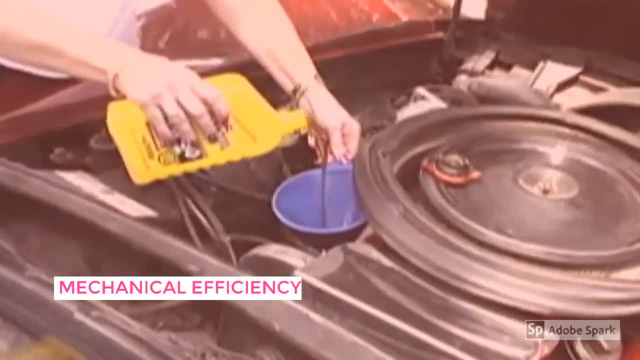 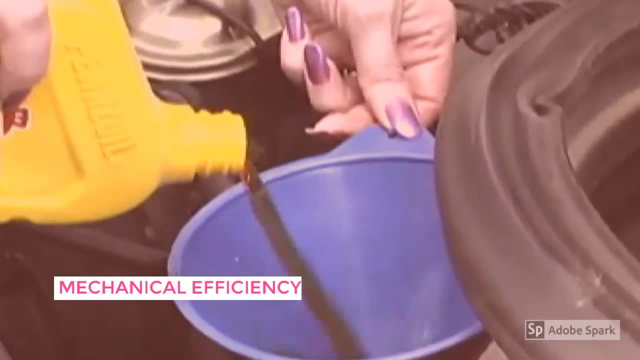 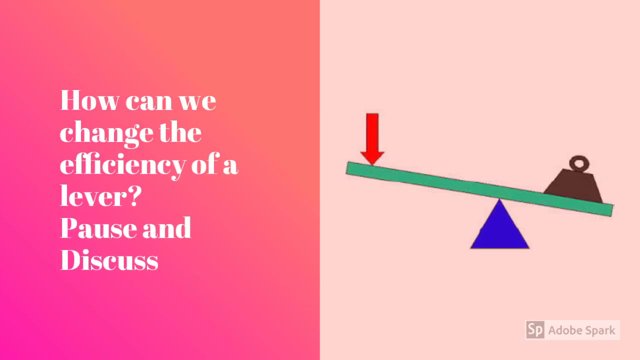 That's why oil and grease are used in machines with many moving parts. The oil or grease will help cut down on friction and help to improve performance and efficiency. How can we change the efficiency of a machine? How can we change the efficiency of a lever? 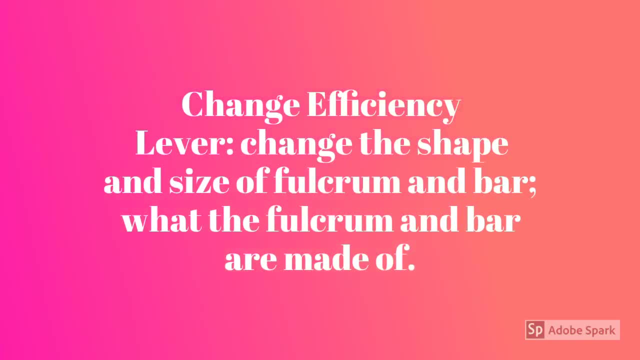 Pause and discuss. You can change the efficiency of a lever by changing the shape or the size of the fulcrum and the bar. You can also change what the fulcrum and the bar are made of the materials. How can we change the efficiency of a pulley?